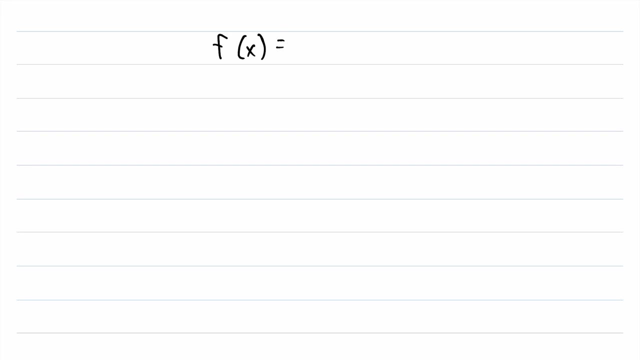 we have two functions. The first one, f of x, is equal to x squared plus 6x minus 2.. And the second function, g of x, is equal to 5x plus 4.. And let's say that we are asked to find f plus g. 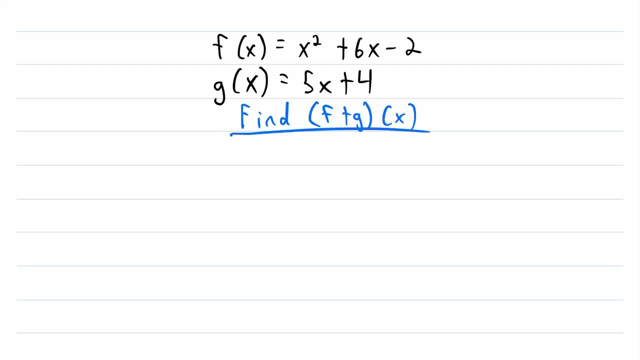 of x. So what does this notation mean? How do we find f plus g of x? Well, I think that this notation is pretty intuitive. f plus g of x is really just shorthand for f of x plus g of x. So to find f plus g of x, all we have to do is add the two. 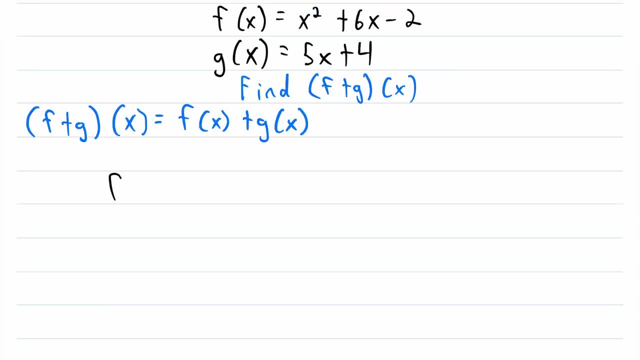 functions f and g together. We are looking for f of x plus g of x. We know that f of x is equal to x squared plus 6x minus 2.. So this here is the function f of x. Then we just need to add g of x. 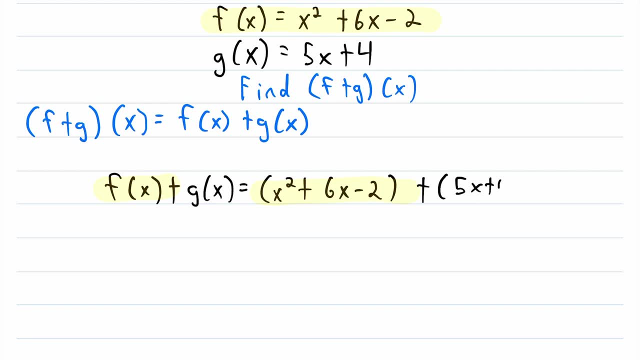 We know that g of x is equal to 5x plus 4.. So that right there is g of x And this right here is f plus g of x. It's f of x plus g of x. So that right there is g of x And this right here is f plus g of x, It's f of x. 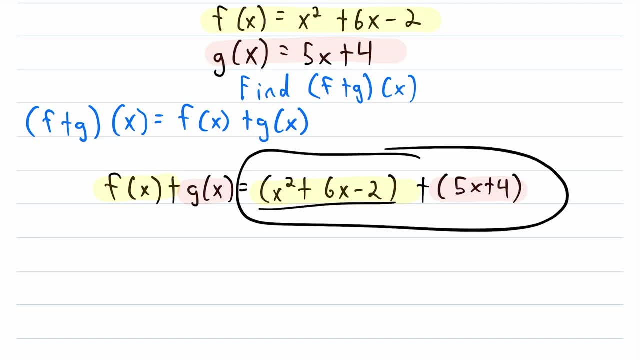 f of x plus g of x, But of course, we're usually going to want to simplify this, So let's go ahead and start simplifying. For starters, neither of these groups is being multiplied by a number or raised to a power or anything like that, So we can begin by. 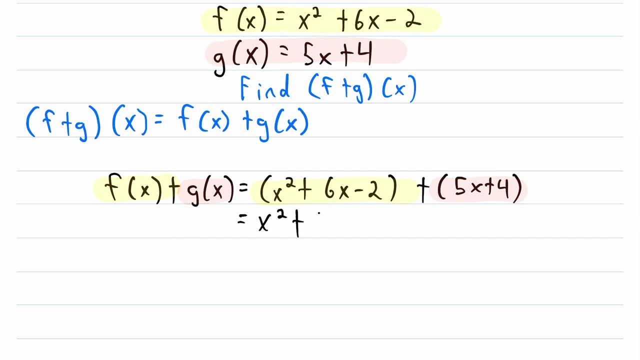 dropping the parentheses. So we have x squared plus 6x minus 2, plus 5x plus 4.. Now all that's left is to combine like terms. If we start by looking at x squared, we see that there are no like terms that we can add x squared to. Then looking at 6x, 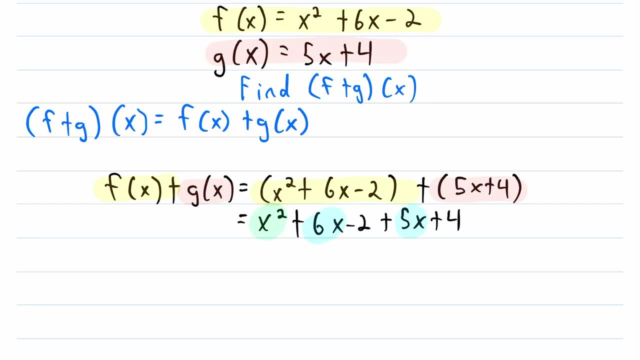 we see that we can add that to 5x. Those are like terms. And then we have minus 2, which we can combine with the plus 4.. Those are both constants. So finally we have x squared plus 6x plus 5x. 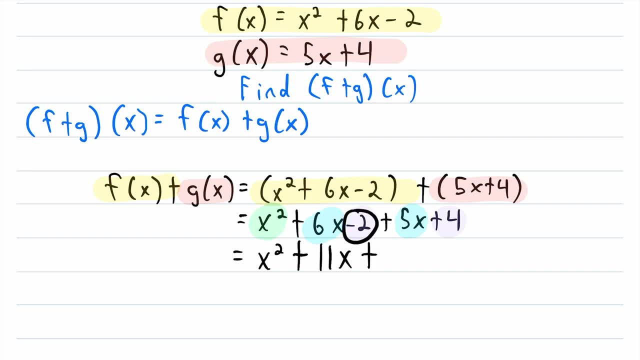 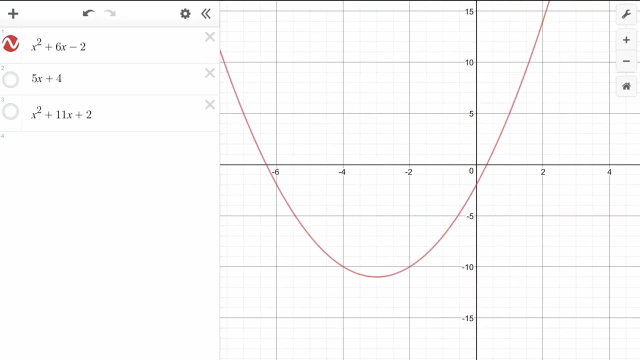 That's just 11x Plus negative 2 plus 4.. That's just positive 2.. So we have plus 2.. And that's it. This is f plus g of x Of x. If you're curious, here's a graph with all three functions In red. we have f of x.